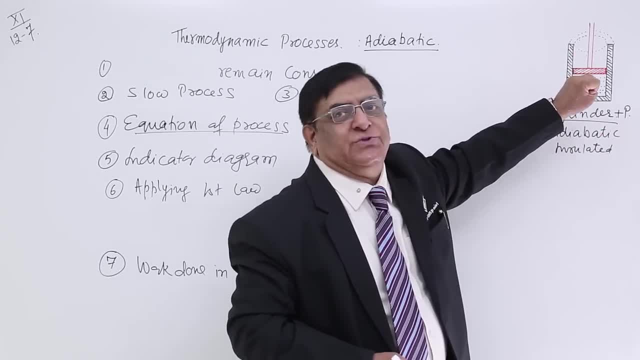 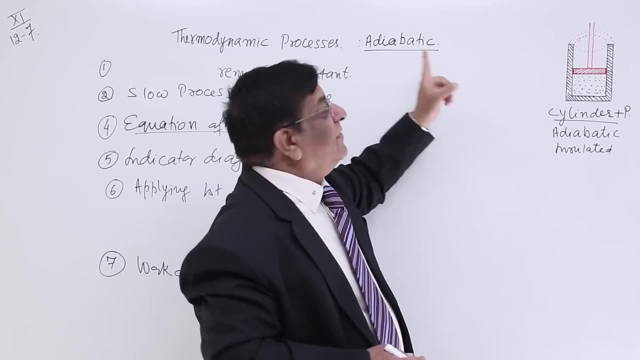 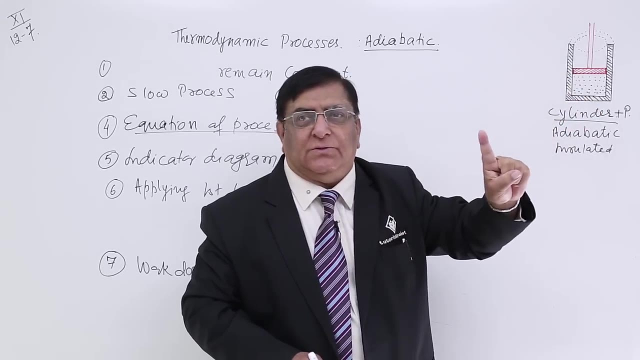 during all this? what type of material we have used here? So here what we want to keep constant, so that it is known as adiabatic Answer: the heat content in the system should not go out and it should not allow from outside to come in. 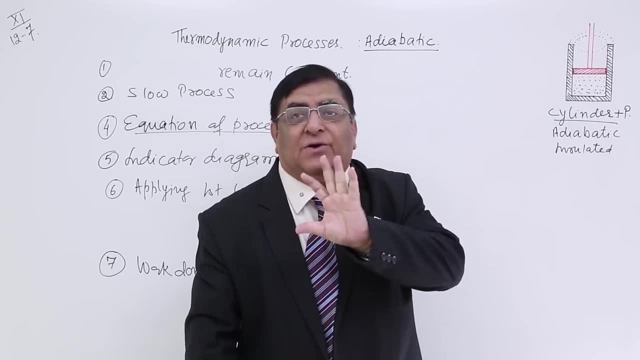 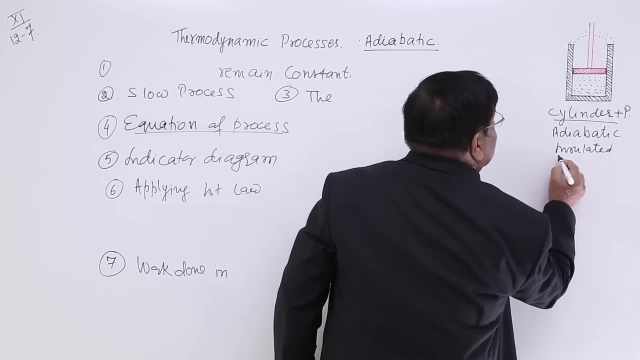 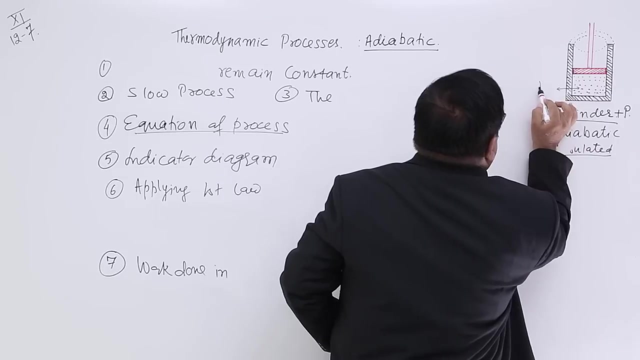 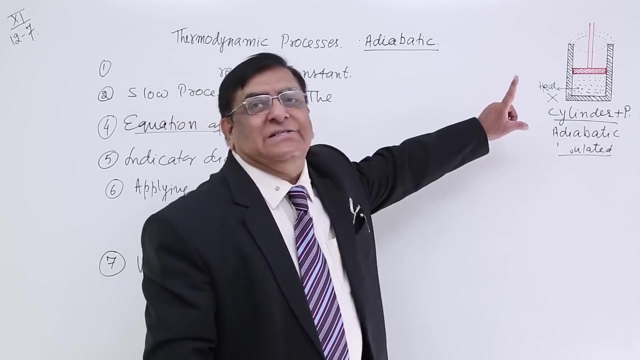 So heat transmission is not there. Therefore we use a cylinder and piston Which is adiabatic, that is insulated. If it is insulated, then transmission of heat is not possible, So that does not take place. What are the other things? 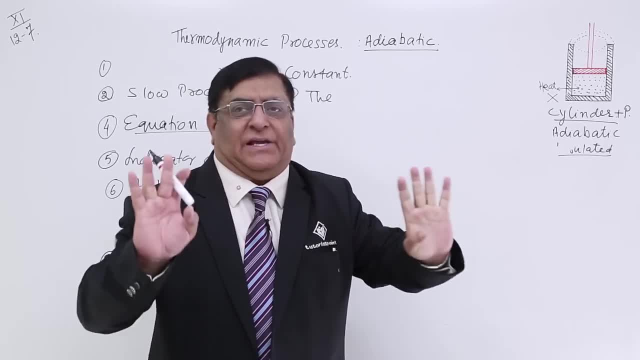 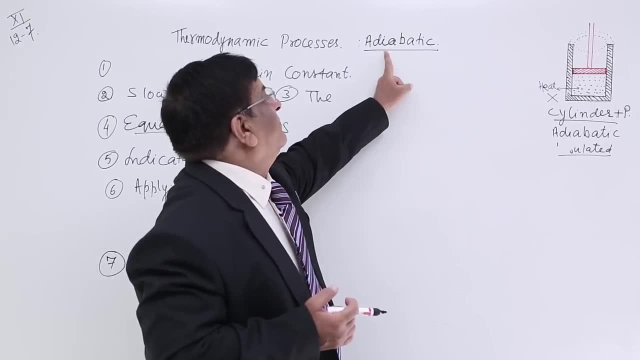 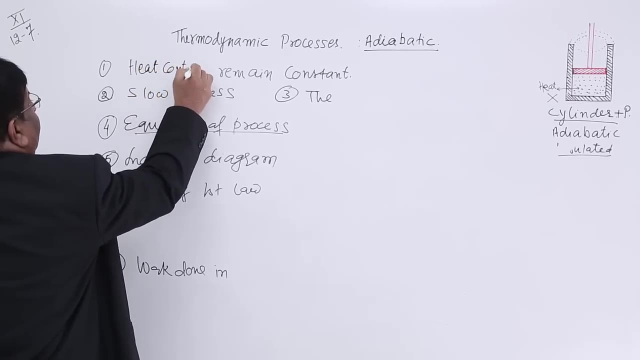 Pressure, volume, temperature, It may change, But what will not change? Heat will not change. If there is such a process, that process will not take place. It will be known as adiabatic. So here heat content remain constant. 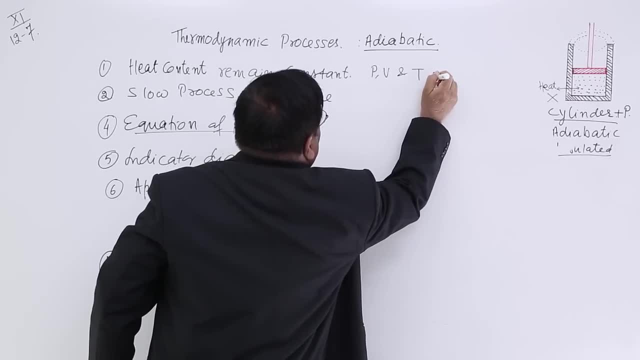 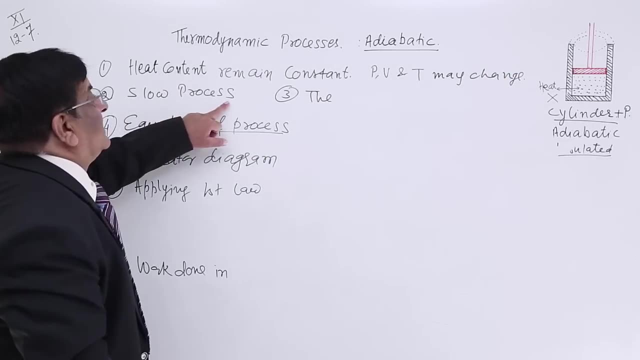 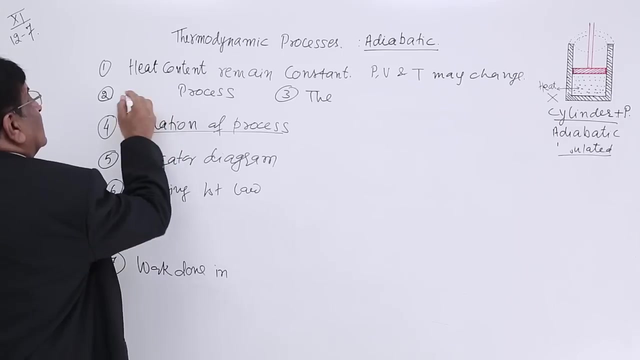 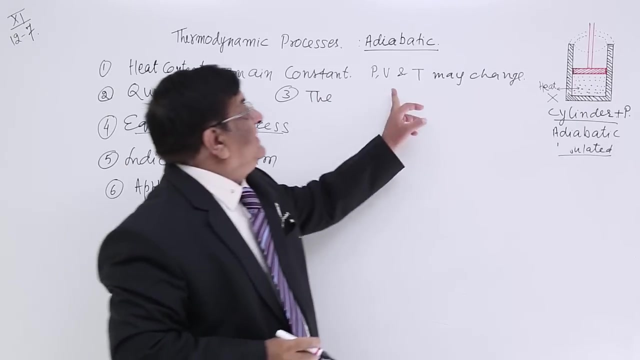 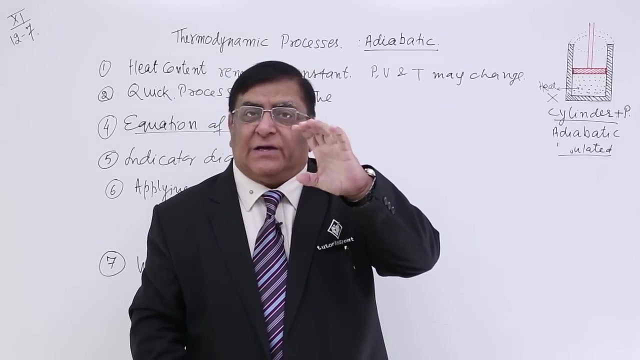 P? V and temperature T may change. Ok then, this is a slow process. no, Invert to isothermal properties. Invert to isothermal properties. Invert to isothermal properties. This is a quick process. We do not during these changes P? V, during the changes of pressure and volume. we want to keep it very quick. So that it does not get time for heat to go out. Whenever the pressure increase, heat will be generated. When heat is generated, temperature will rise And because the temperature has risen, the heat will try To go out By the time it goes out. before that, again, there is a expansion. 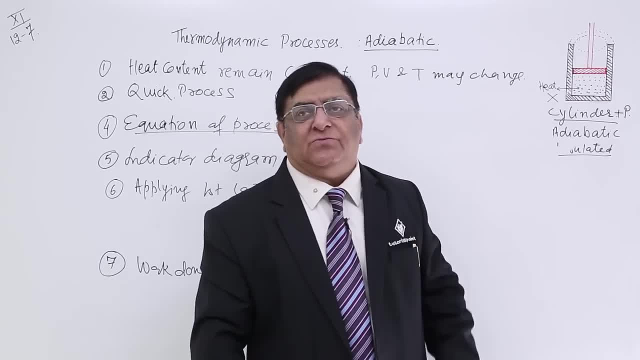 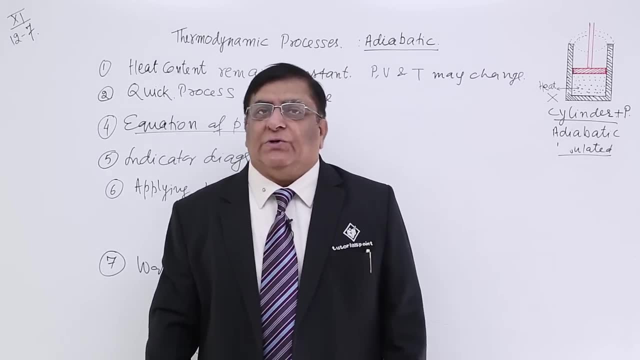 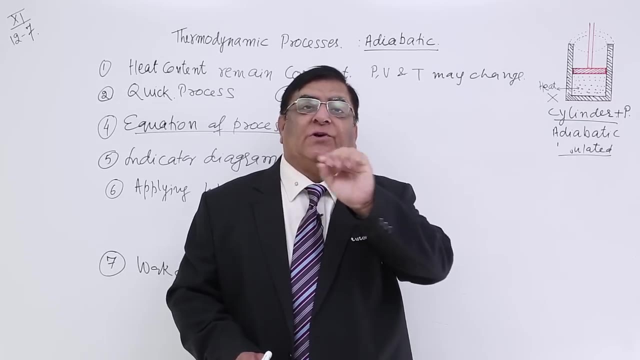 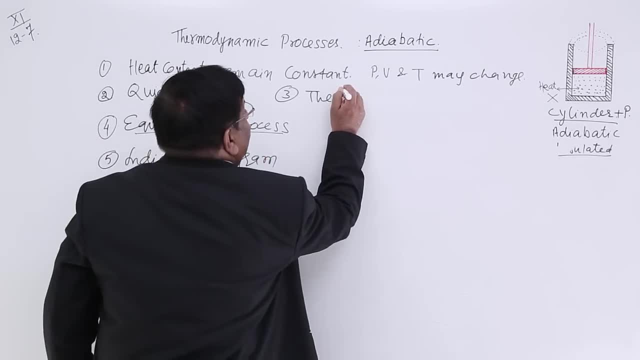 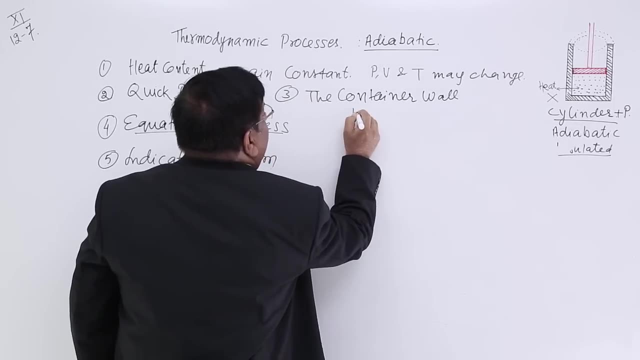 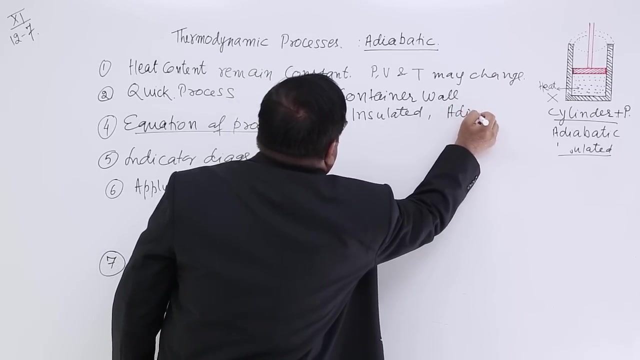 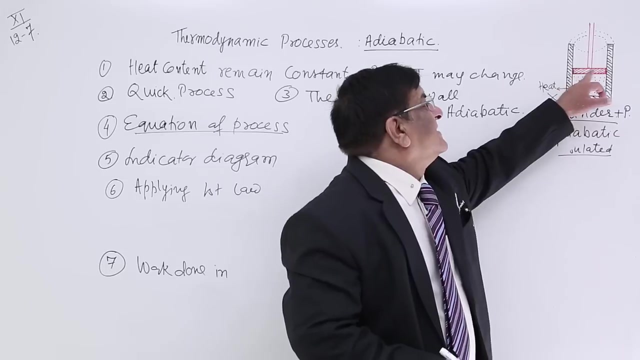 How is the container, The container wall, The container wall is insulated, And what do we call such wall in thermodynamics? Adiabatic wall. So the walls means from all the sides, including piston. everything should be insulated, adiabatic. 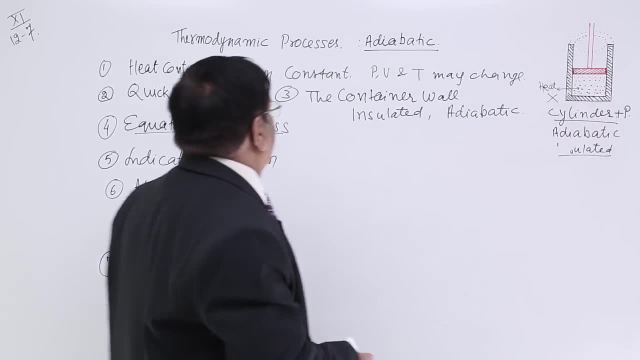 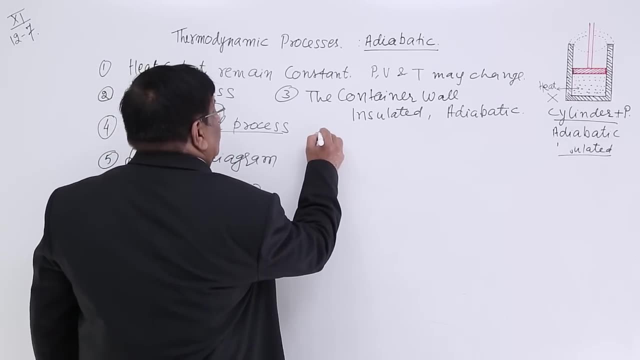 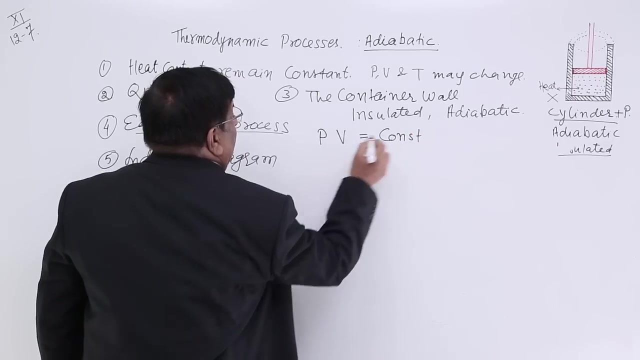 So that heat cannot go out. So the walls, means from all the sides, including piston, everything should be insulated. adiabatic go out, it will not leak out. Then equation of this process, the equation of isothermal process was P into V as constant. But in adiabatic we find that P and V to the power 1, 1 is. 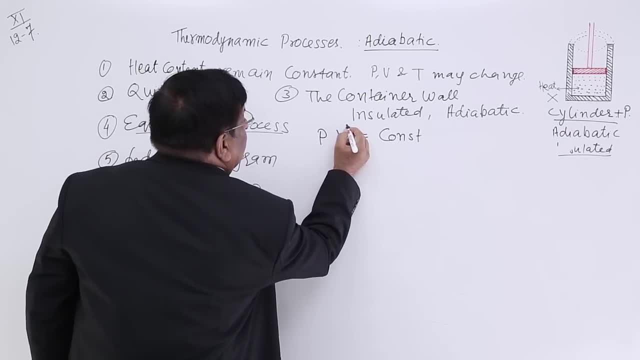 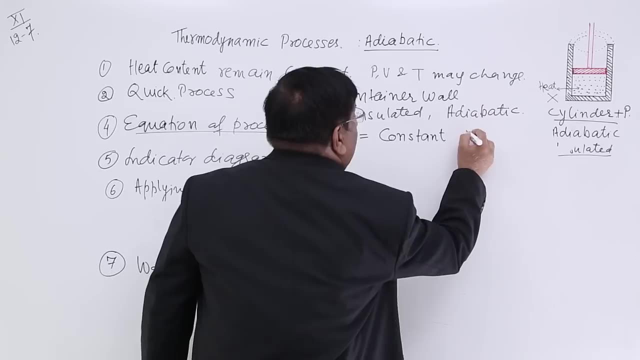 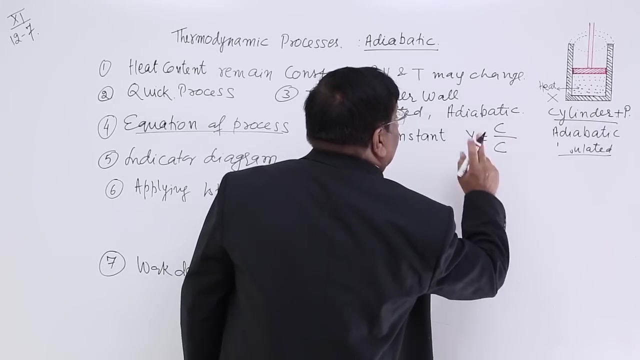 not there Here. P multiplied by V to the power, gamma is constant. What is this gamma? So gamma is ratio of two specific heat of the gas, Which are the two specific heat: Specific heat at constant pressure and specific heat at constant volume. The ratio of Cp- Cb is: 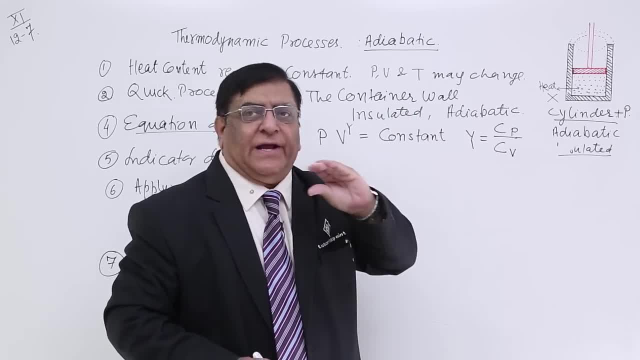 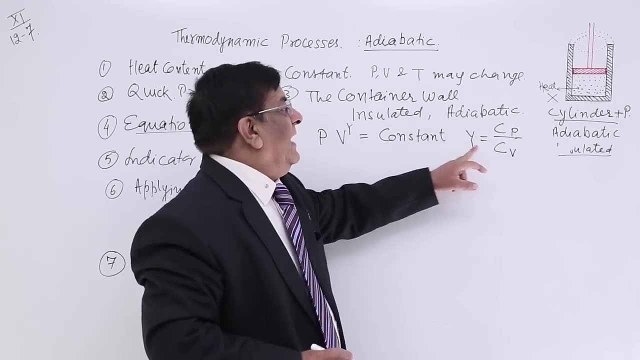 gamma, and that is the constant for every gas. For diatomic gas there is one value of Cp upon Cb, For mono-atomic one, for tri-atomic there is one, And for the diatomic one there is three times the constant of extra and for one the 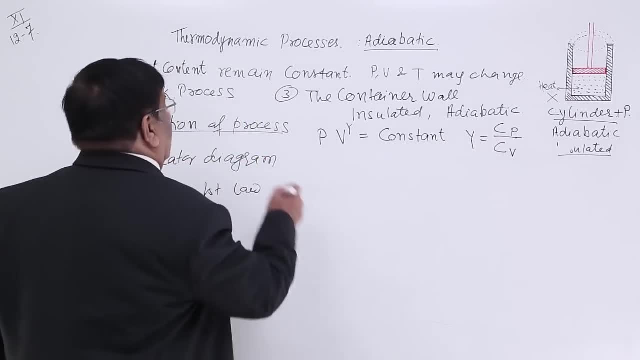 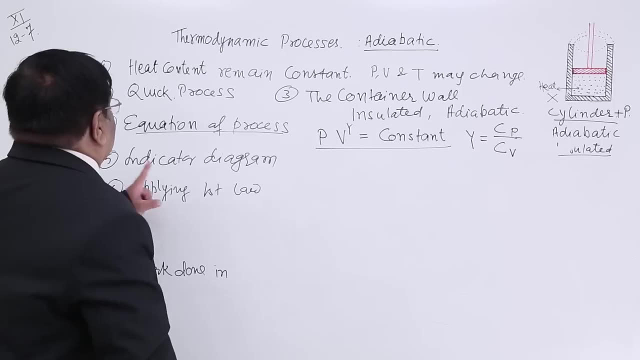 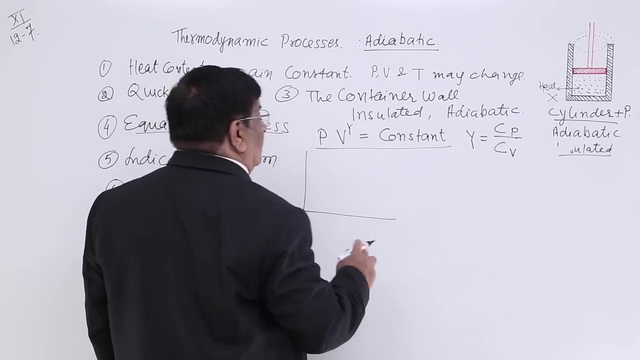 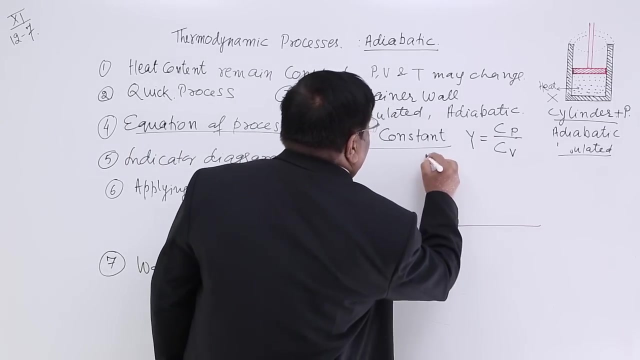 this ratio gives gamma. So the equation for adiabatic process is PV to the power. gamma is constant. Then indicator diagram, Indicator diagram. I make here both the indicator diagram, so that we can differentiate between the two. This is P and V. Again, PV One I will make. 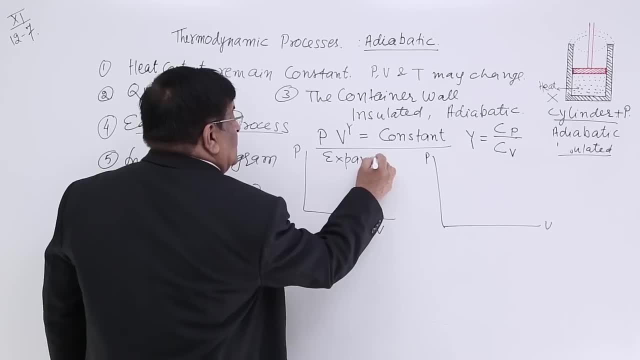 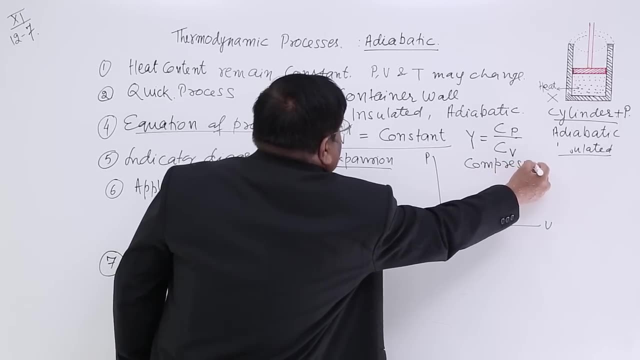 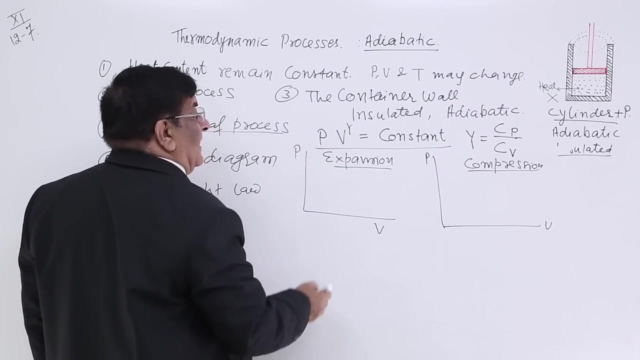 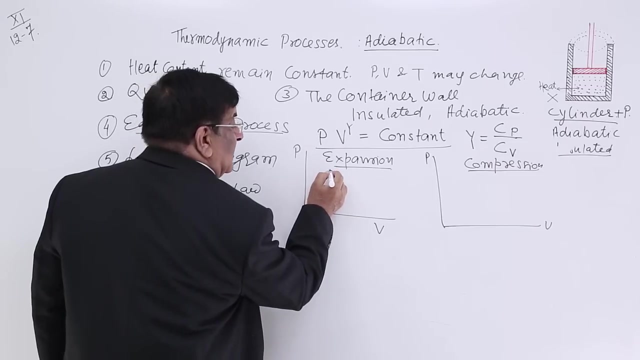 for expansion and one for compression. Ok, In this I make two lines, one for isothermal, one for adiabatic. In isothermal we have already studied when volume is increased, pressure decreased, and this is the graph For isothermal. 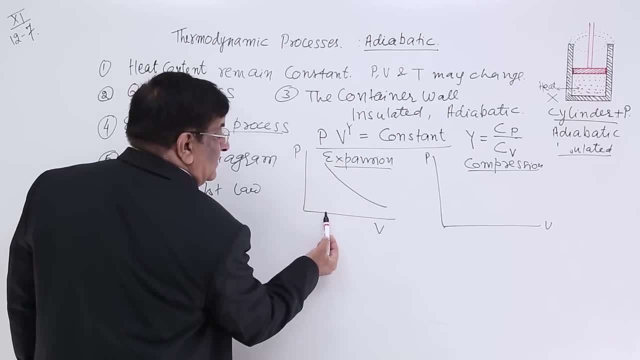 Now volume started less, increased more. that is why we call it expansion. but how to show it? we will put arrow here. this arrow shows the process: start from smaller volume and it has gone to the larger volume. ok, this is expansion, isothermal. now how it will be for adiabatic. 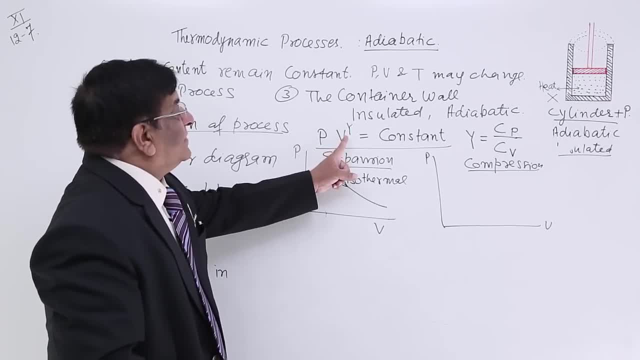 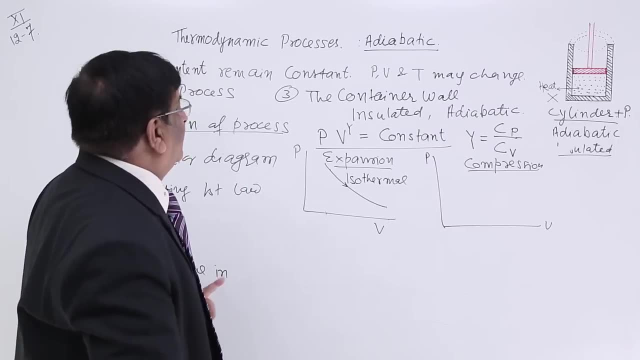 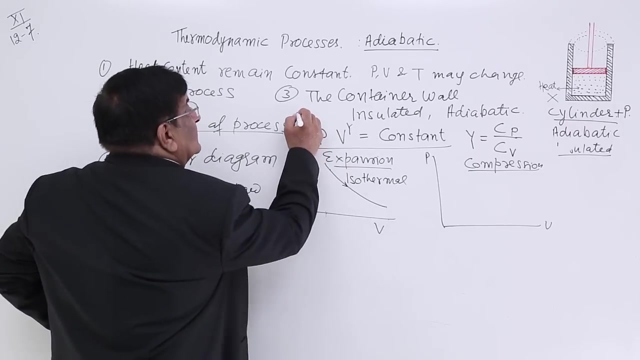 here we find that volume has a power which is more than one. so volume decrease very sharply. volume decrease very sharply in isothermal it was p proportionate to one upon v to the power one, this p proportionate to one upon v, to the power one in isothermal and to the 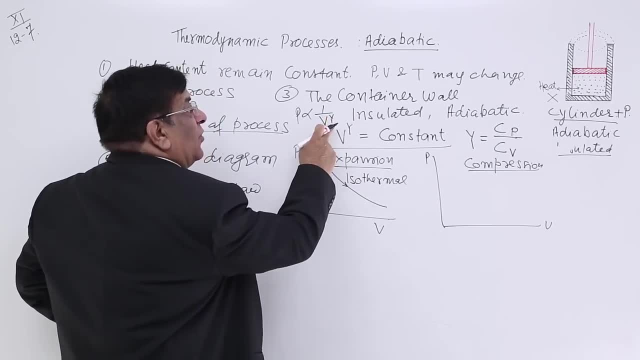 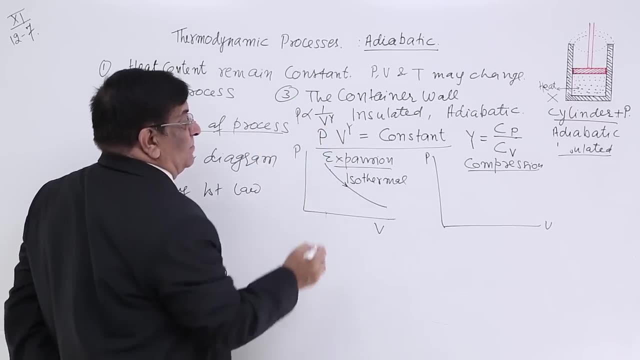 power gamma in adiabatic. so gamma is always more than one. if it is more than one, then it is made to be controlled. for than 1, then P will decrease very sharply. so we get a graph here. This is for adiabatic. 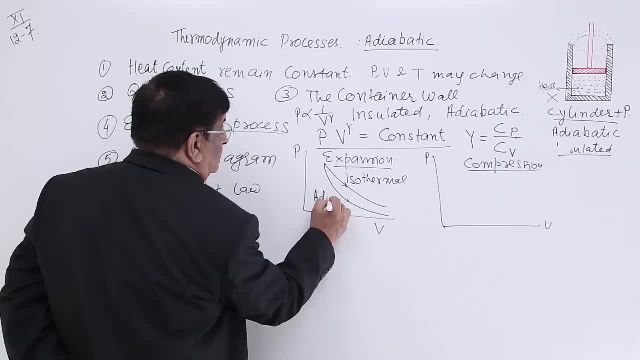 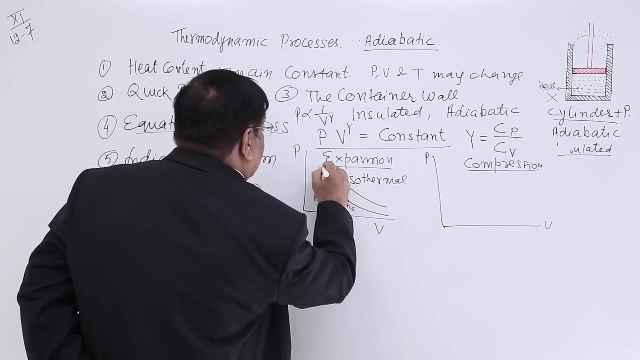 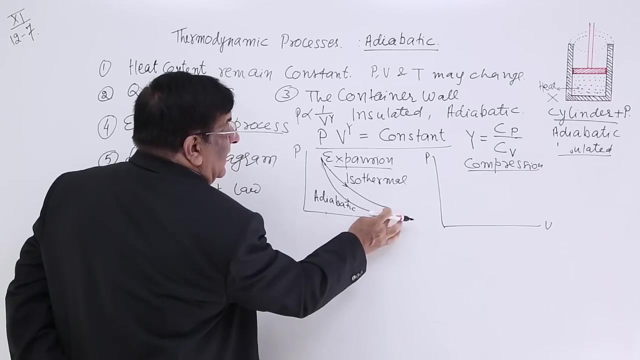 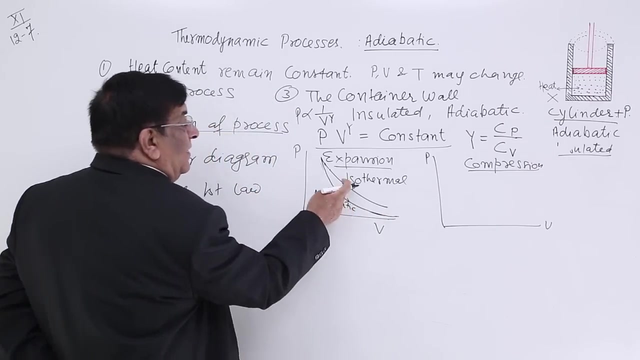 process. So this is graph for adiabatic and I will correct it because it should always be inclined this way. So there should be no doubt. Let us make it this way, Ok, But the slope is more in adiabatic, So please remember this is adiabatic and this is isothermal expansion. 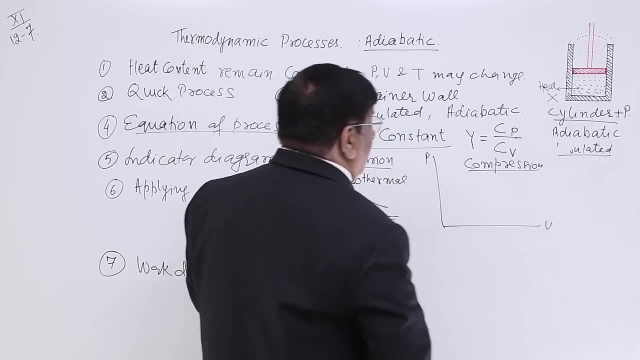 Now in the compression the initial volume is large and when we compress it the pressure increase just by having a small volume. So this is the initial volume. expansion of the 倍 clip ____. the pressure increase just by having a small volume, this time, and then 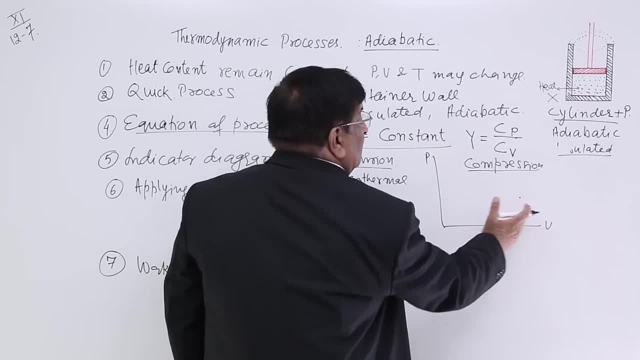 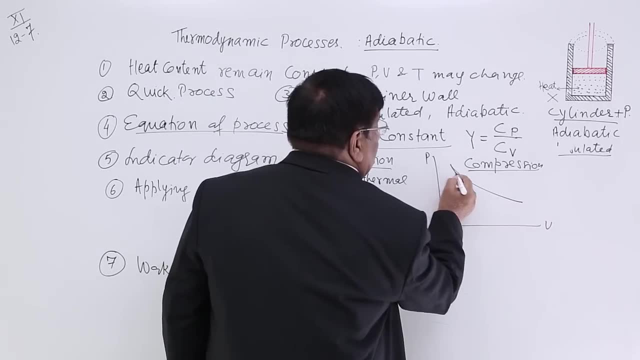 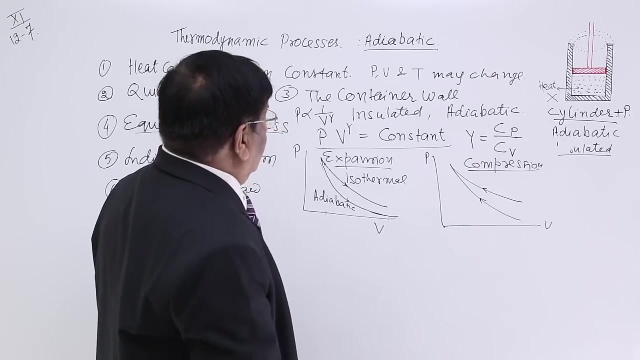 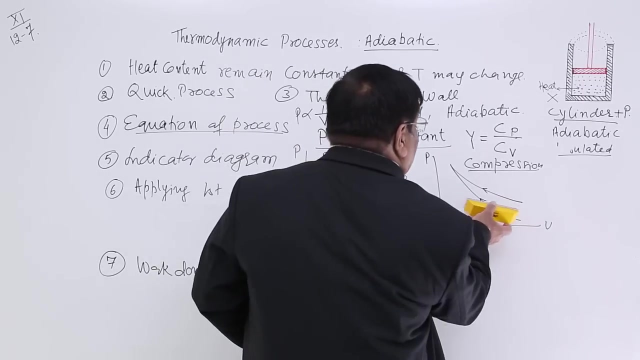 increase the volume decrease. Pressure increase, volume decrease. And here we have these two graphs: One is this and one is this. Which one is the one? Here again we have this is R. Let us make it the other way. Let the starting point be same. That is one. is this one other? 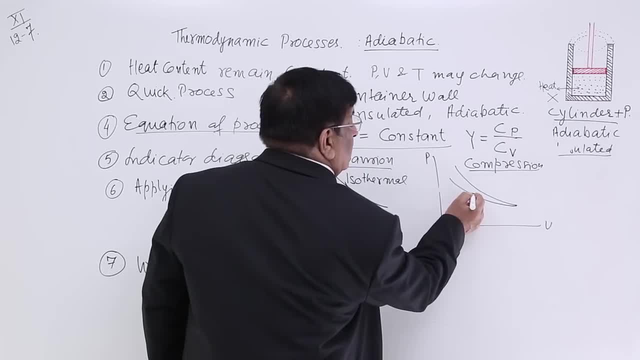 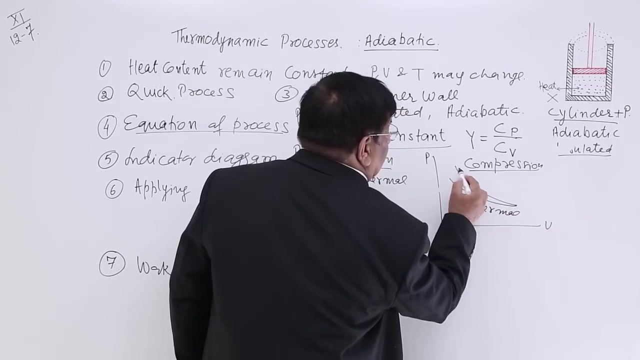 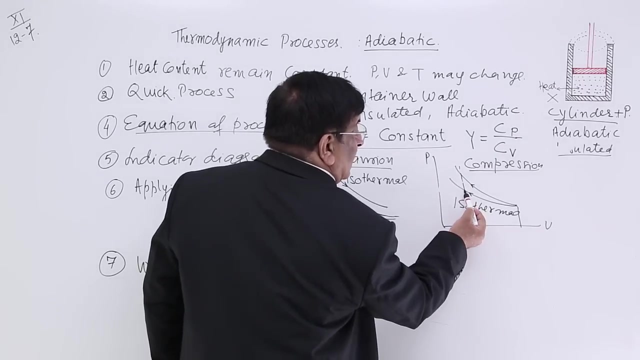 is this one Here which has got larger slope. This is slope fast, Increase fast and this increase slow. So this is isothermal and this is isothermal, And here for a small change of volume. you see, for change of volume, this pressure change. 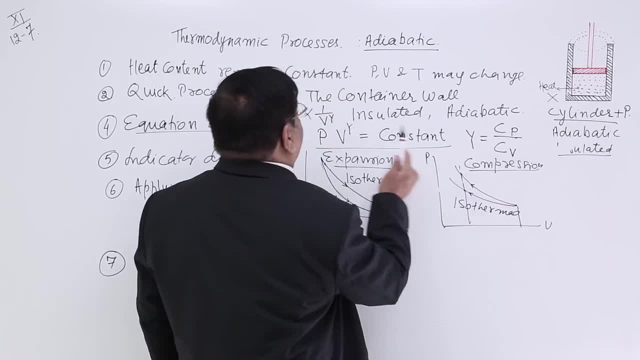 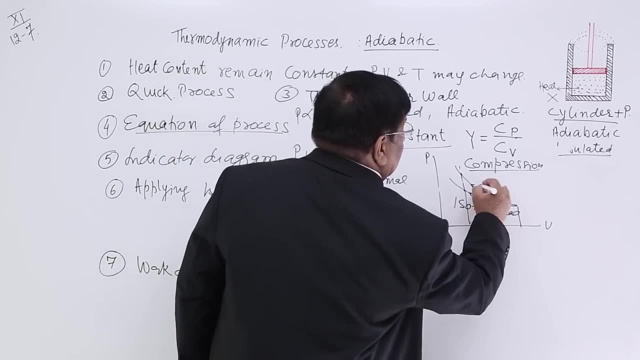 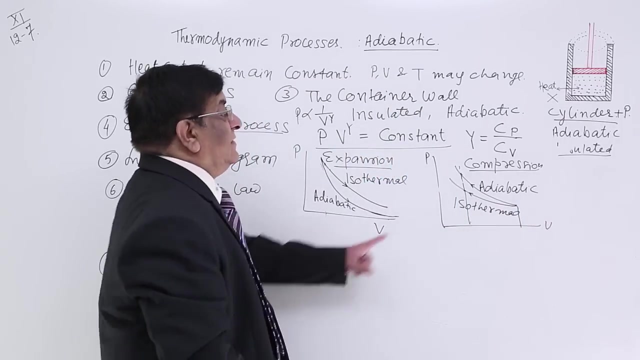 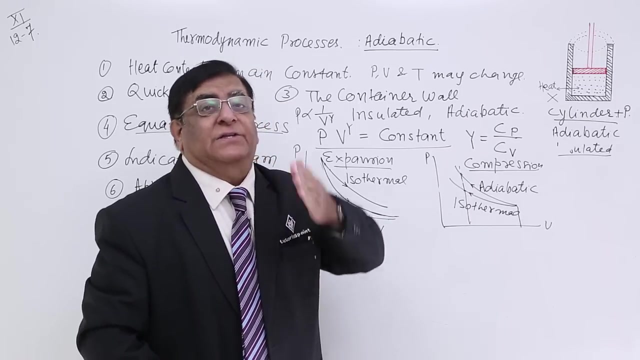 is small, this pressure change is more And we know that where pressure change is more with the volume, that is adiabatic. So this is adiabatic and this is isothermal, this is for compression, But in both of them one thing is common which you should remember, That is the slope, The 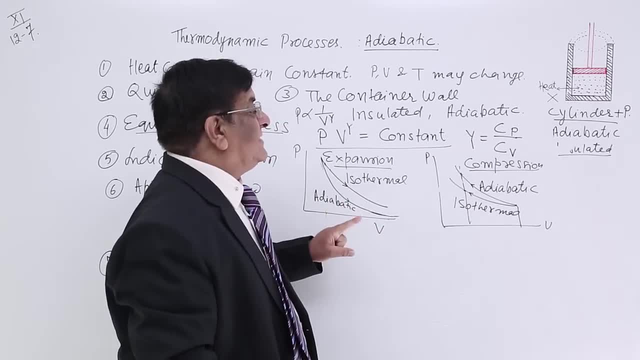 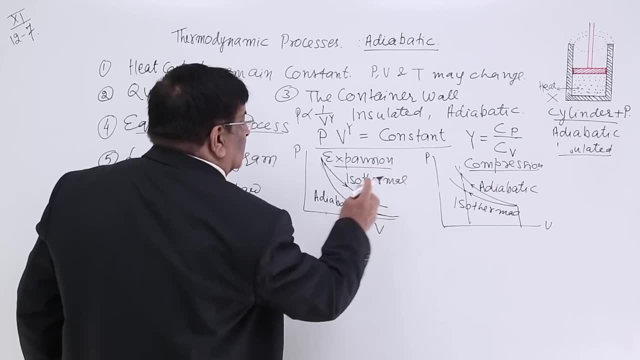 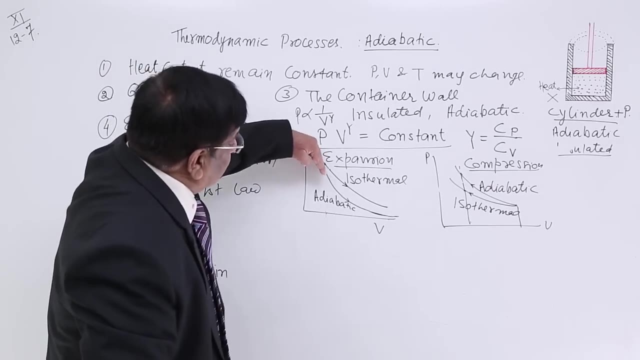 slope is more in adiabatic Slope is less in isothermal. Whether it is expansion or compression, it appears reverse, because here is the starting point, here is the starting point, Doesn't matter, This slope is large Here. this slope is large, So larger slope. 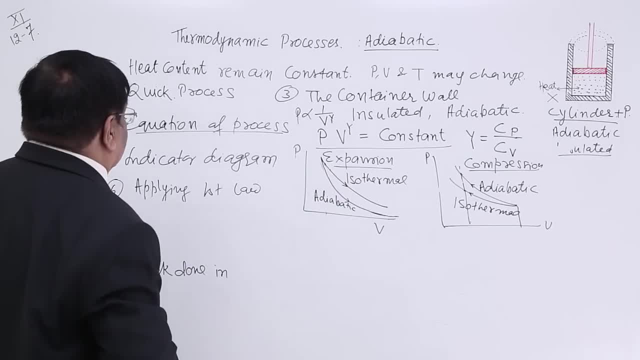 adiabatic. Okay, These are the indicator diagram. Then application of first law. The application of first law of thermodynamics that says that when heat delta Q is given, it is change in internal energy plus work done. This is first law. This is how the heat is used Now in. 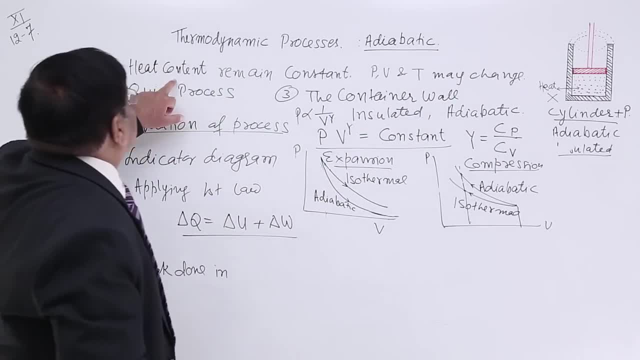 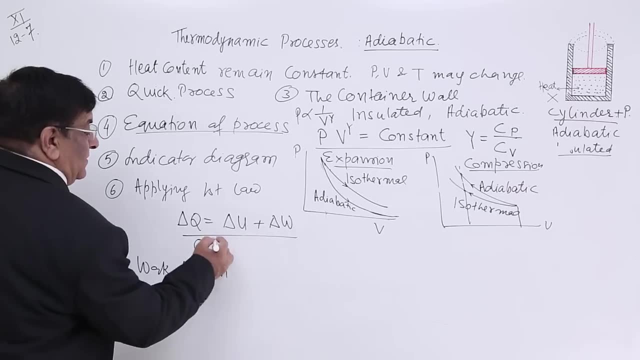 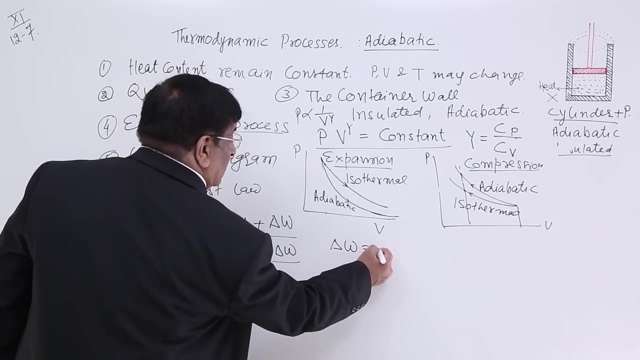 adiabatic. what does not change. The heat contents remain constant. So the change in heat is 0,. no change is equal to delta U plus delta W. Now this gives us one thing, that is, delta W is equal to negative of delta U internal. 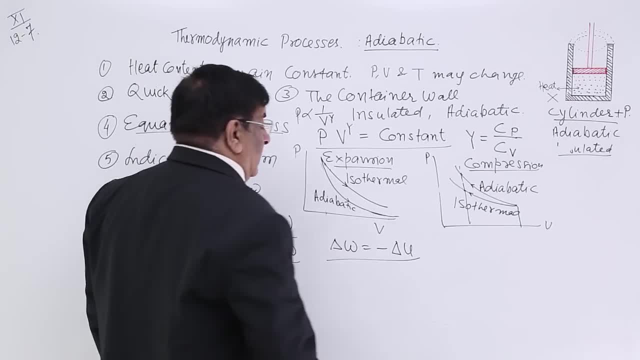 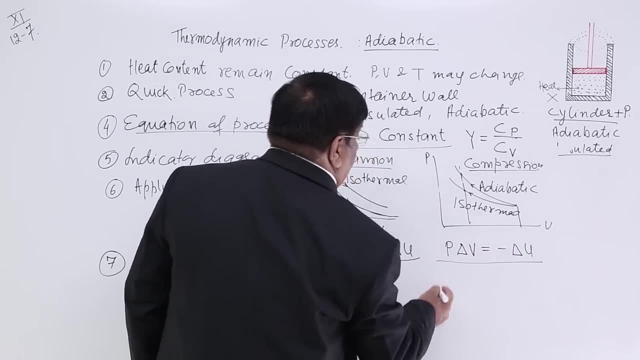 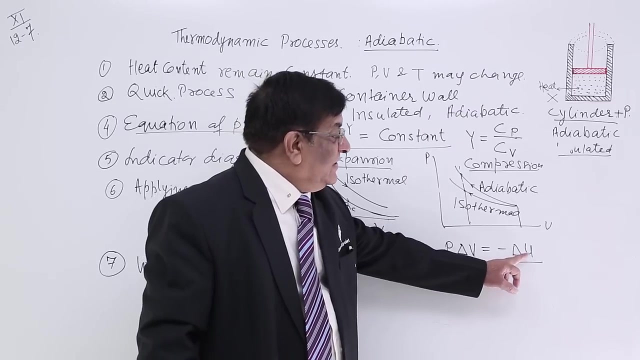 energy. What do we write? delta W, equal to Delta W is P, into delta V is equal to, so minus delta u. What does this mean? How do we know that internal energy has decreased? The indicator for change in internal energy is its temperature. If internal energy increase, 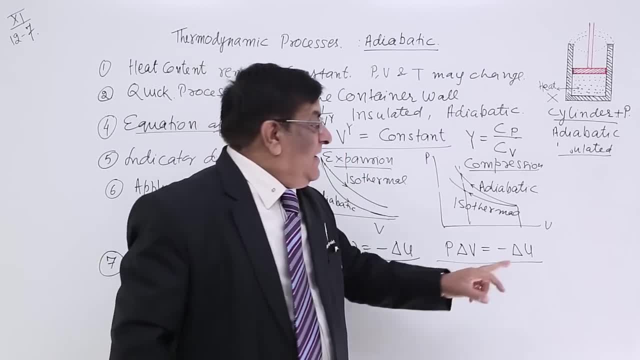 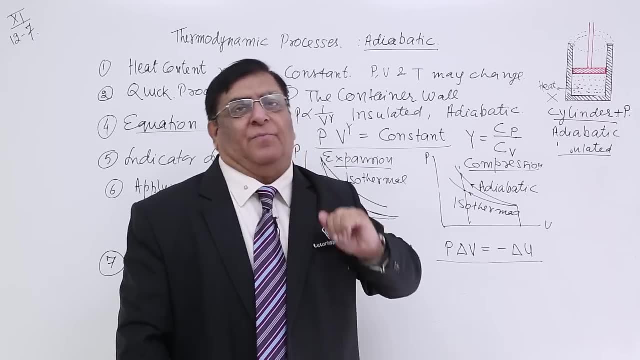 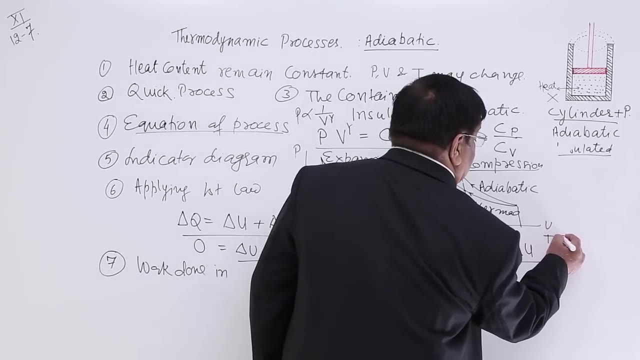 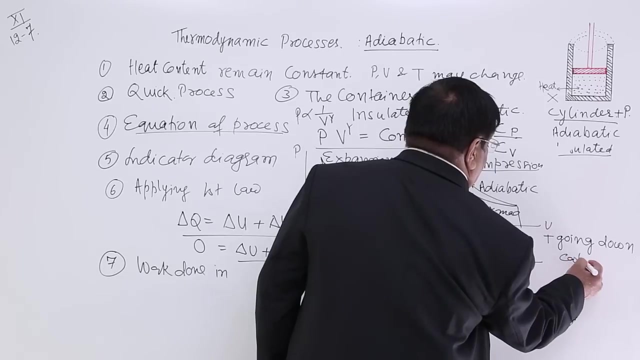 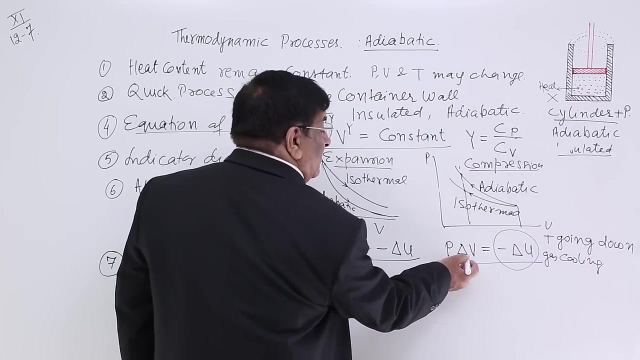 positive, the temperature is increasing. If internal energy is negative, that means the value is coming down, that means temperature is coming down. So this says the gas is cooling, T going down and the gas cooling. What when this happens? When there is a p into delta. 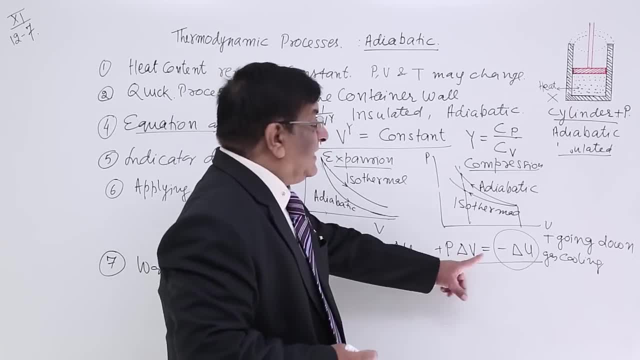 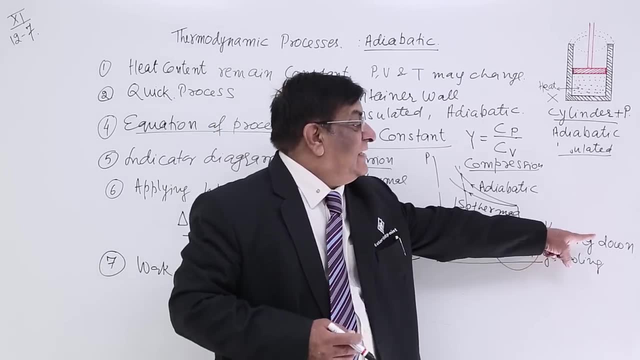 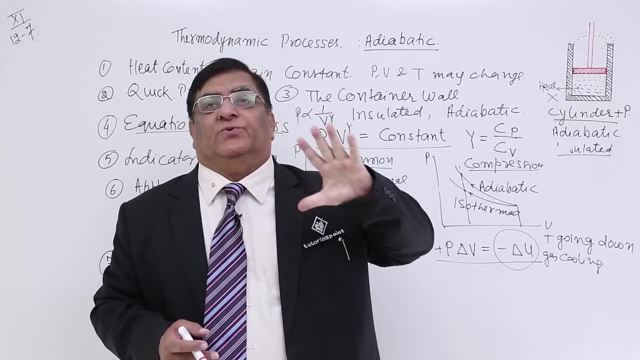 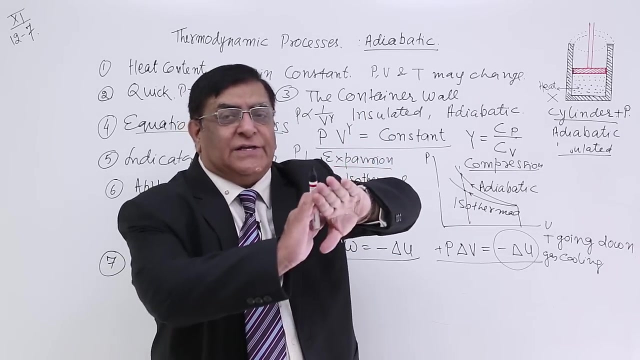 v. positive Positive delta v is what Increase in the volume. Whenever there is a increase in the volume, the temperature goes down in adiabatic Process. Whenever there is increase in the volume, temperature goes down. Want to see this? Have air in your mouth. It is at a temperature of 37.. Your body is at a temperature of 37. 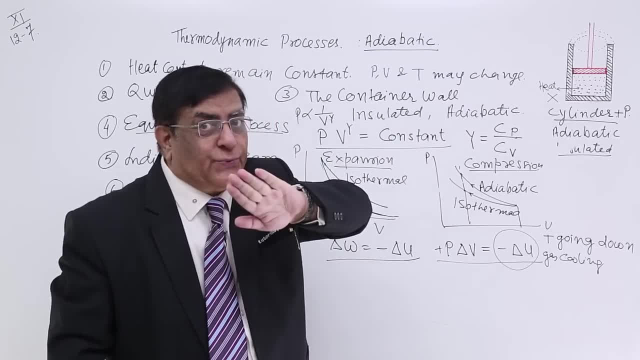 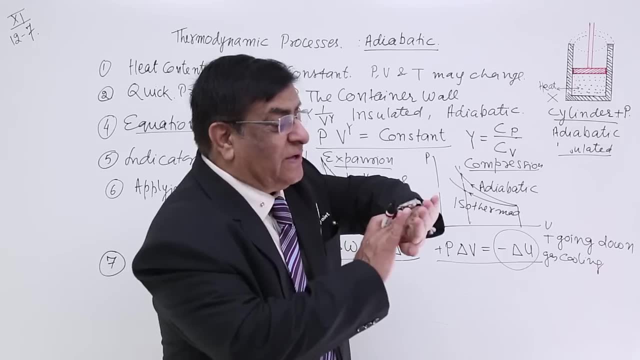 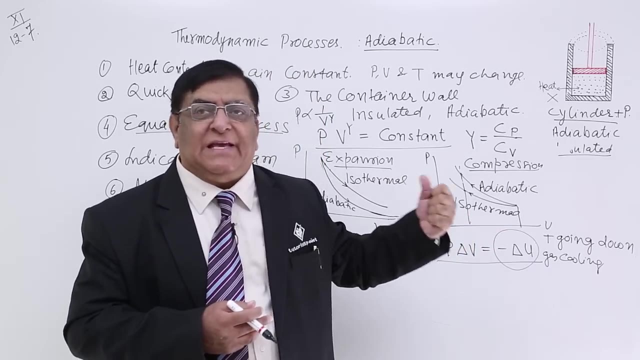 and make it. If you make this, the air expands, The volume increase. What happens to temperature? It goes down. That is why you feel cool here. So that is example of getting cooling. The same thing happens in refrigerator. In refrigerator there is expansion Inside. 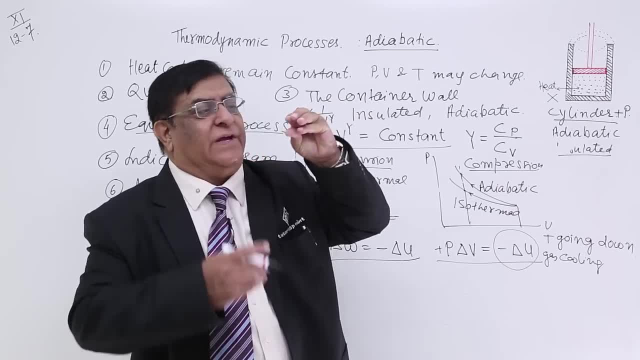 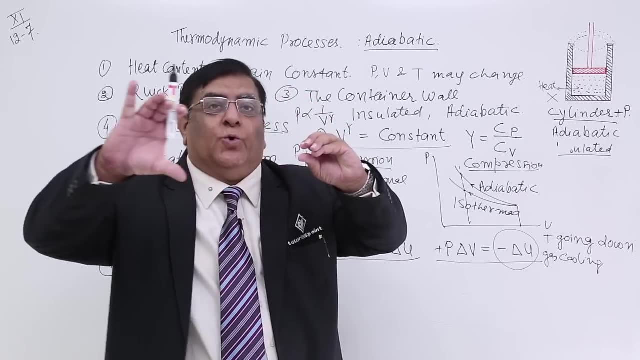 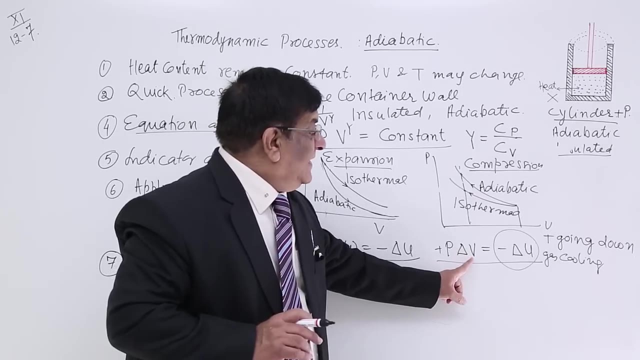 the freezer. the gas comes through a capillary tube, very small bore, and suddenly it is allowed to expand in a larger bore tube. So the gas goes like this: The volume increase many times. When the volume increase, there is a fall in the temperature and it become very cool. 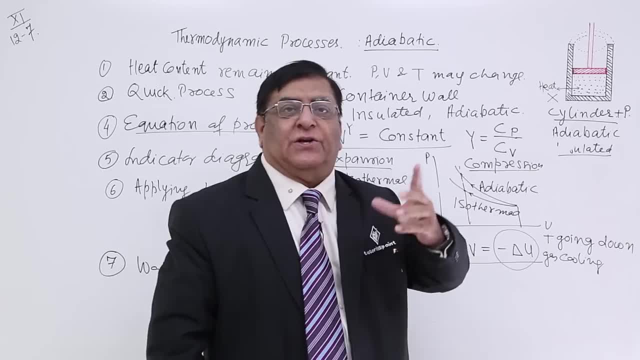 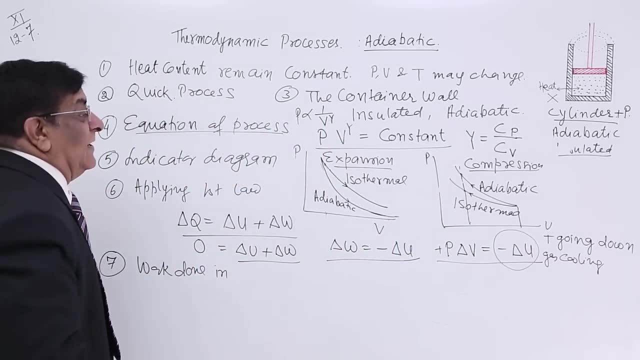 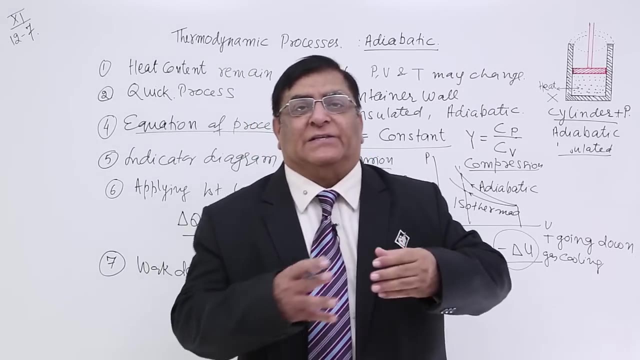 Less than 0 degree. And that is how refrigeration, air conditioning, all these machines are work on this principle. This is adiabatic expansion. So what is the cause of cooling? Adiabatic expansion is one cause of cooling, Wherever we expand it. Suppose a tyre bussed out Then 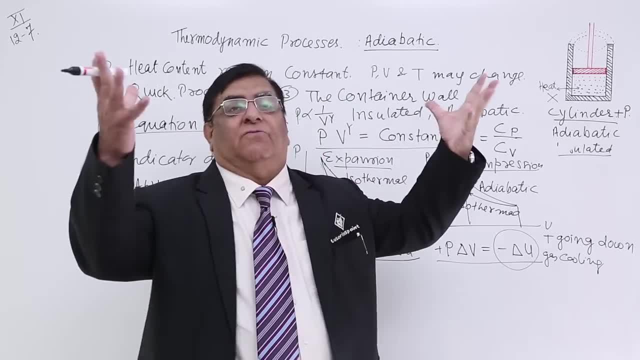 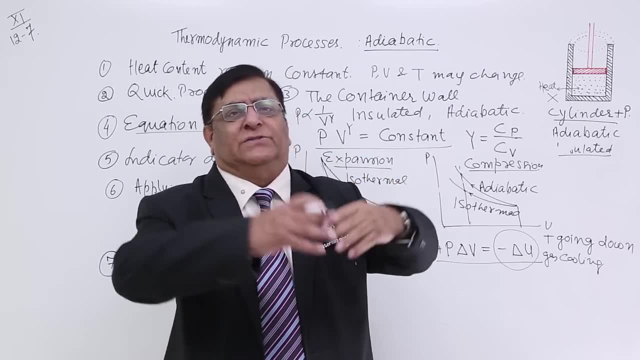 suddenly all the air molecules, the volume increase. When the volume increase and their temperature will go down, the air goes down. The air will go down Then when it is pressed down. of course we do not feel it, because air mix up very fast. so this is application of